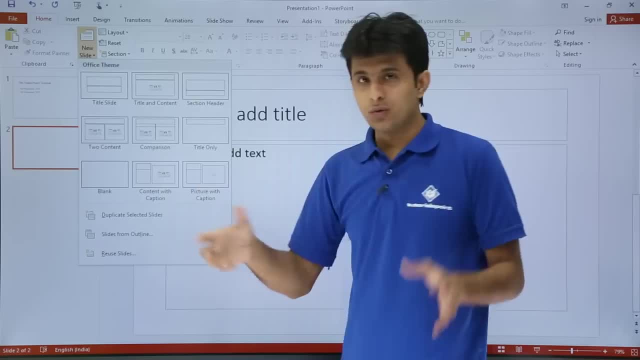 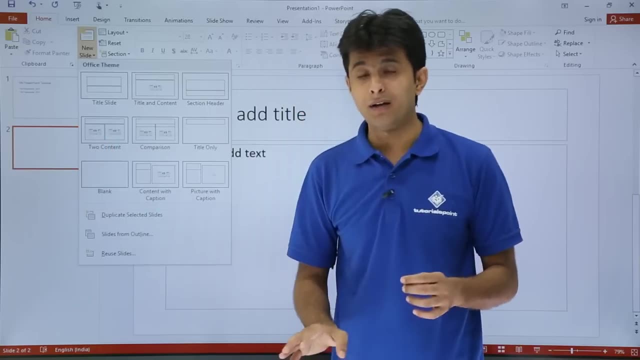 only want a title, you can select this option. and if you want to compare two different charts or two different tables, two different photographs, Etc. You can select this comparison and so on. So, based on your requirement, you can choose. which type of theme do you want? So I'll select this comparison. So you see, I can just keep on writing here. 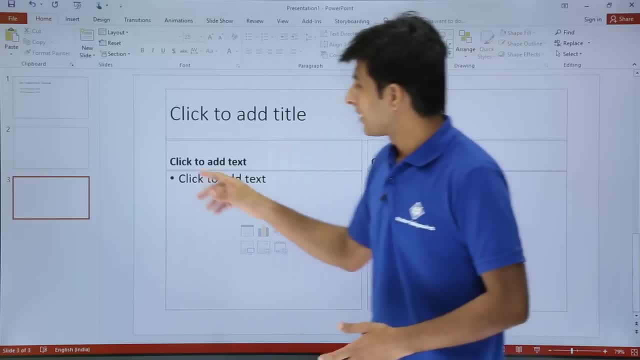 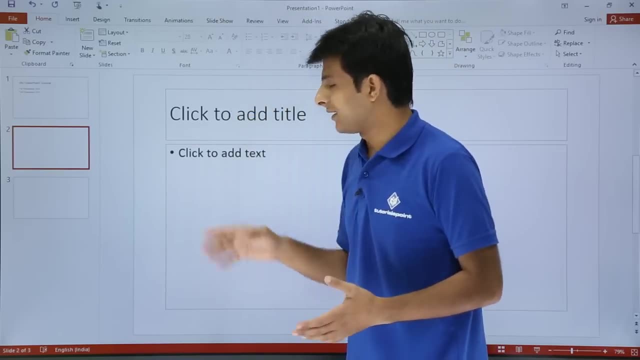 something. I can paste two images or I can compare like that. Similarly, suppose I'm on the second slide and if I do not like this kind of slide, which is the theme which is available here- title and heading the contain, If I want to change it, what you can do is you can go to this home tab On this. 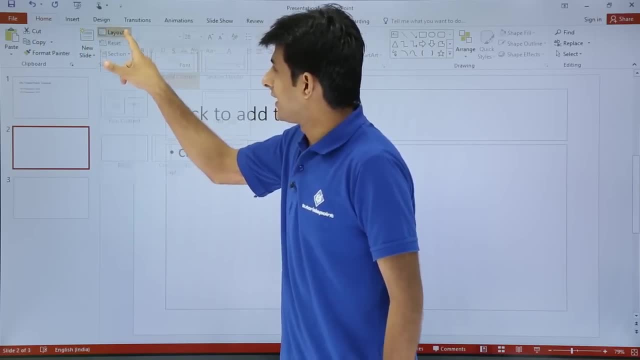 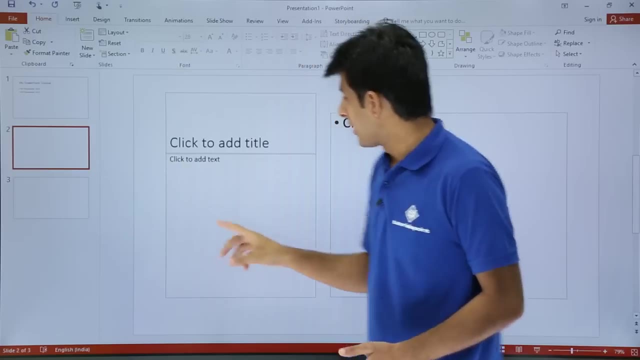 place. you have slides group available Here if you see there's a layout. So layout whichever is available, you can change it to some other layout. So I'll select this. contain with caption. So I'll click on that. So existing layout is existing theme which is changed. 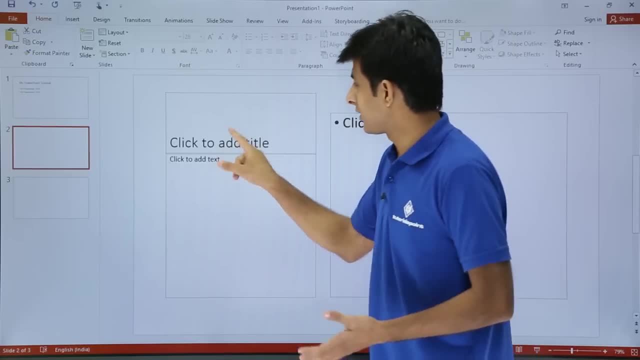 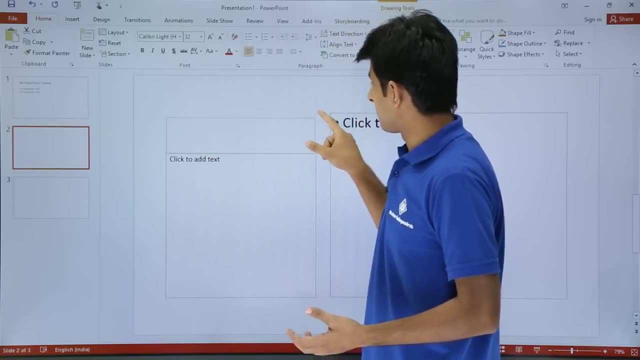 by this contain and layout theme right, So you can keep on customizing and then you can keep on typing whatever is required itself. If you do not like this one, if you want to bring it back, suppose this this: I have changed it by mistake while writing. I have changed this one. I have changed. 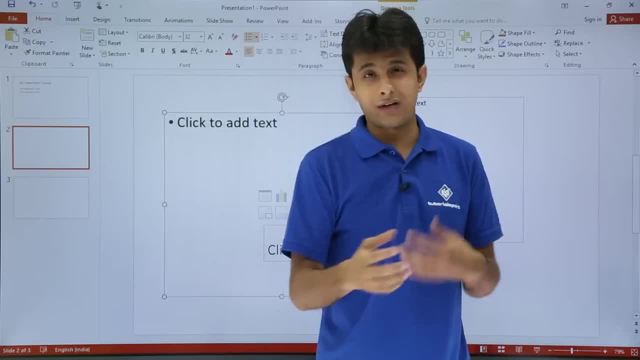 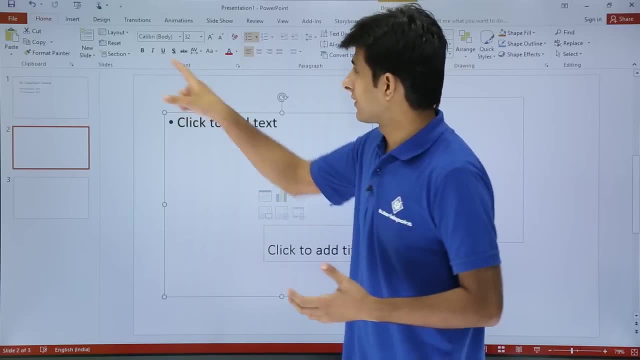 the position of this contain. I have changed the position of this contain. You try to- you know- experiment different areas. You try to experiment different areas. You try to experiment different areas. You try to take it to that place. But suppose if you want to bring it back to the original place, you can just 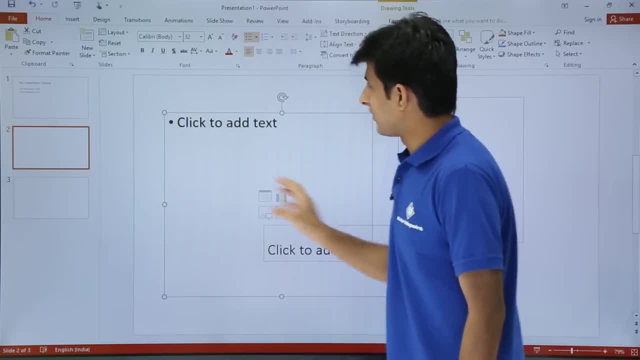 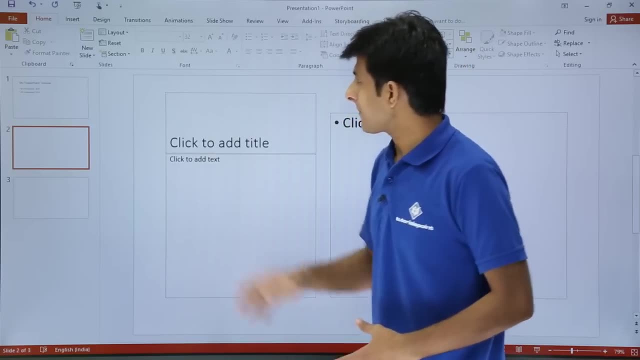 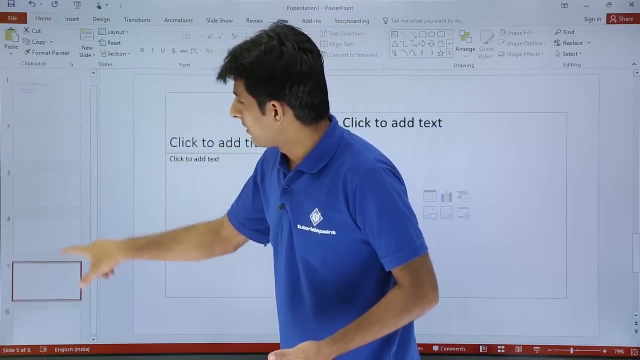 click on this reset button. This reset button. once I click, see what happens on the screen. Click on reset. It will come back to the original position which it was available at the prior place, right? Second one is: if I have three slides and I keep on creating multiple slides, right Now, I remember. 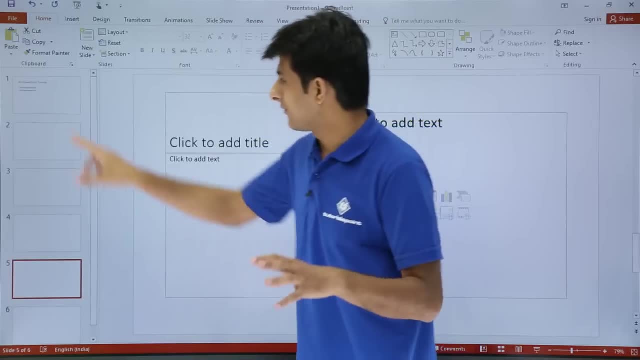 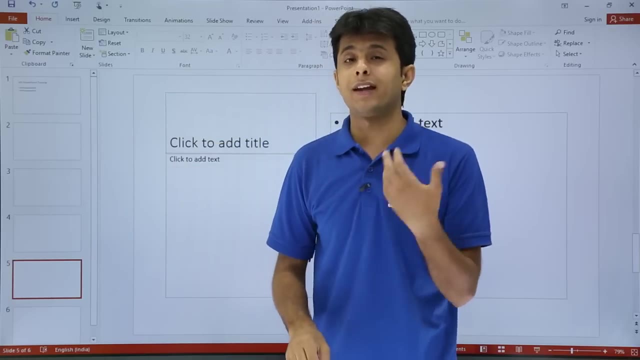 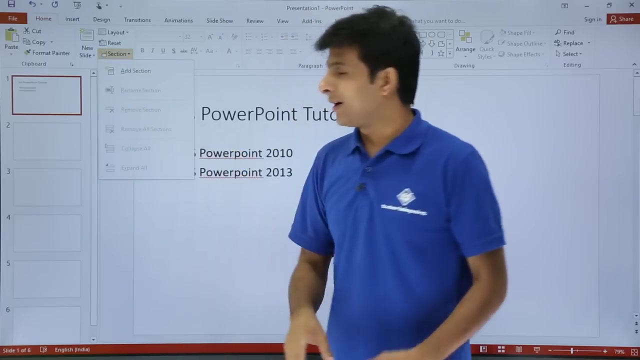 when I go for a presentation I have four slides, or let's say I have three slides, which is for myself. These three slides, I can make one section and I can group it. I can name the group of that section. How do I do that? I'll just keep my cursor at the first slide and go to this section, part and. 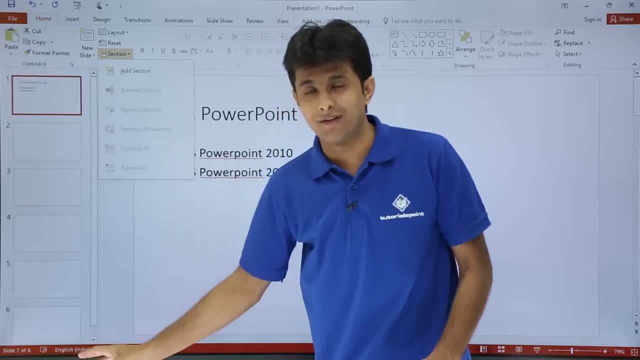 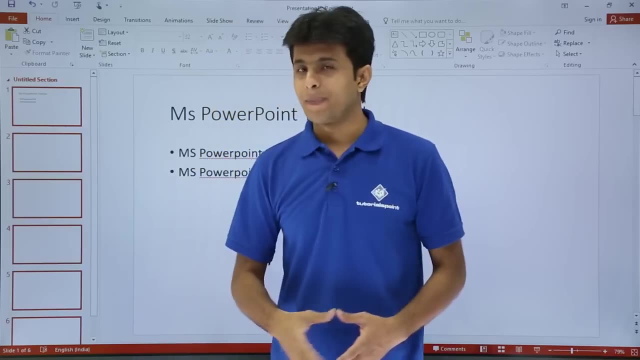 I can say as add a section. So these are sections for this slides available. It makes our work easy when we go for a presentation, So I'll just click on this add section. You see there's an untitled section given here, So all the slides belong to this untitled section. Now what I'll do is: I want. 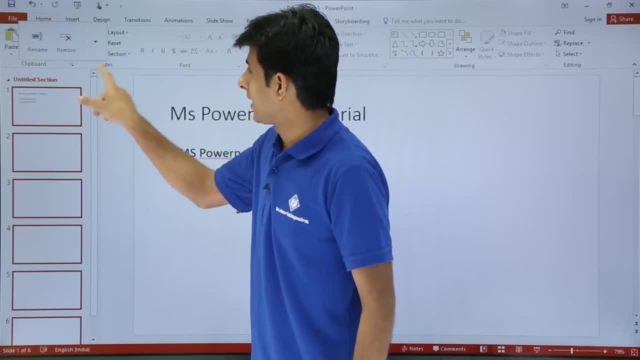 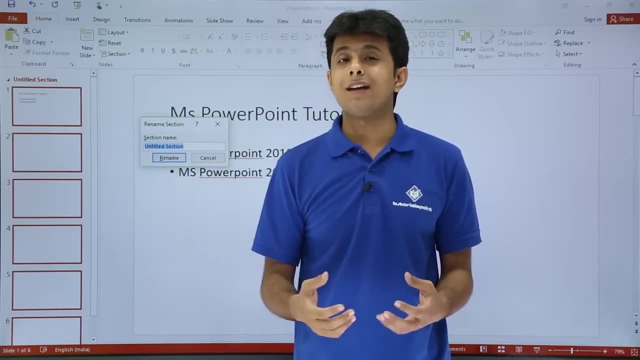 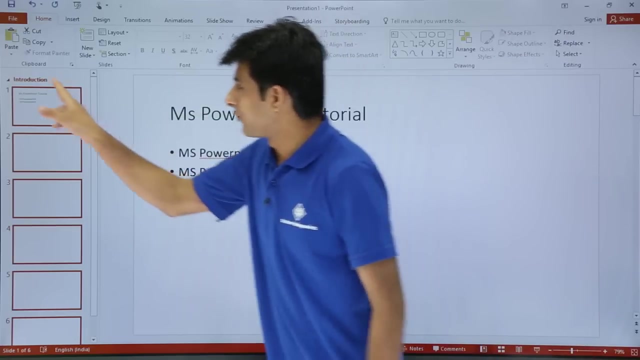 to change the name of this untitled section. So I'll click on that thing and I can say a section. so now, what name do I want to give it? So this is the dialog box: Untitled section. I will say as I want to do as introduction. So I'll type here: as introduction, Click on rename. So if you observe, 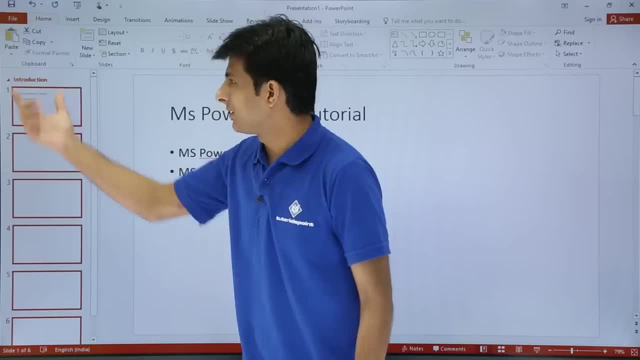 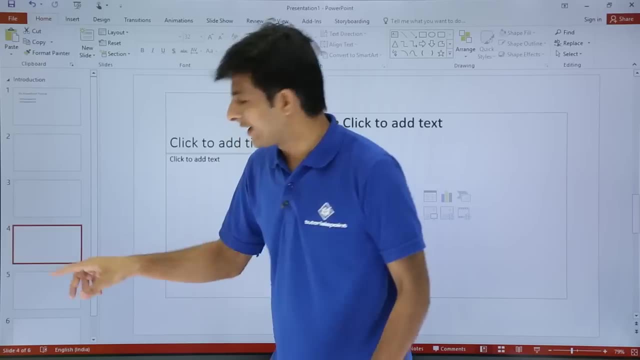 all these slides, whichever in that you know that place that has been into the group. that is what you call introduction. That's a section created Now I want. I want to create, after fourth slide, some other, let's say body presentation, So I can just click, keep my cursor at the fourth slide. 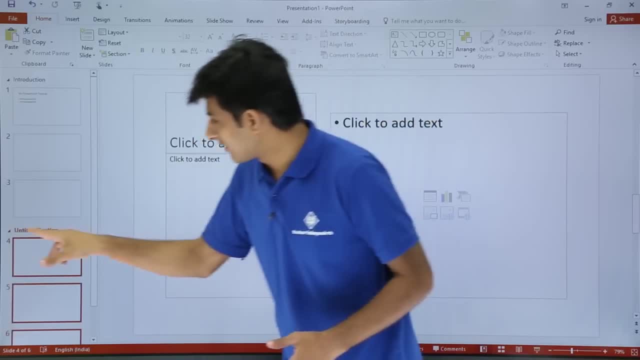 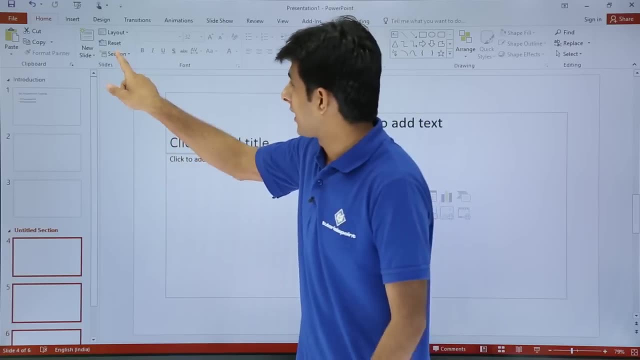 and go to this section and I can click on this add section. So if you see there's an untitled section, again the name has changed. Now I want to say as body presentation, or I can see as body of the presentation, I can say I can just go to the. 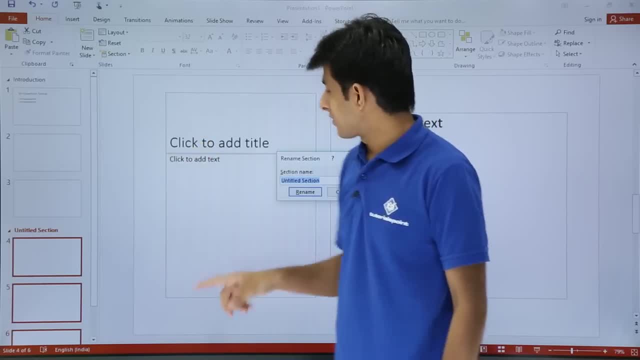 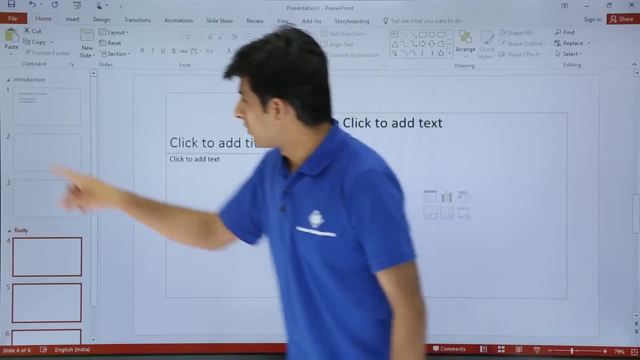 section and I can click on this rename section, Rename section. again a dialog box will come. I can start typing, I can say as body like that, and I can click on rename. So I'll just minimize that section like this. I'll just keep my cursor over here and I can minimize that section Similarly. 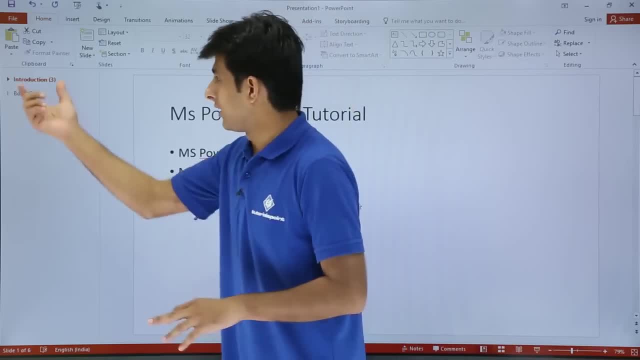 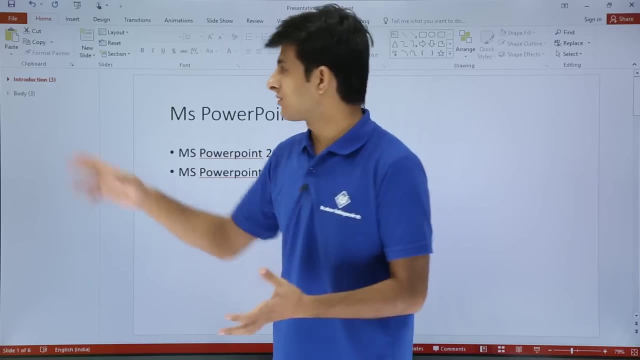 this section I can minimize. So it says there are three slides into the introduction, There are three slides into the body section. So accordingly you can work on that and when you go for a presentation- suppose you have missed some part- you can immediately navigate to that place. 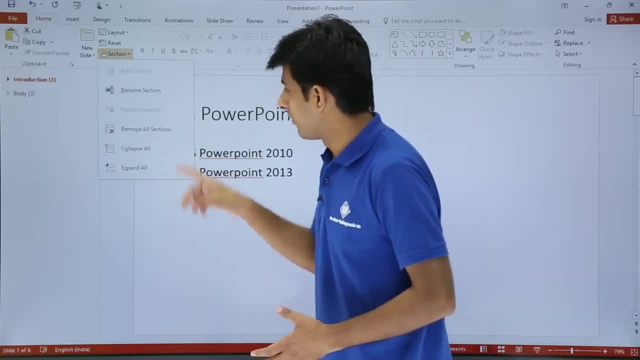 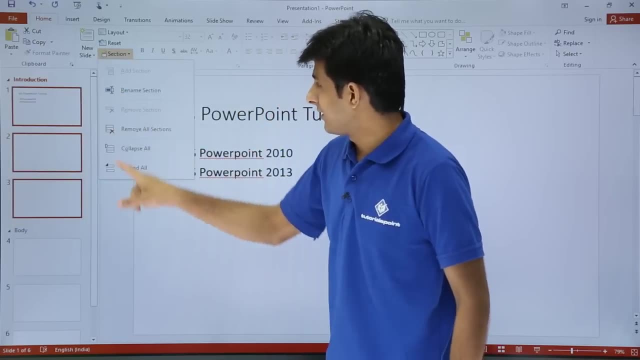 right. Similarly, there are various options available, like remove all sections, collapse all and expand all. So if I say, expand all, you see, all the sections will be expanded. If I say, here I want to collapse all the sections, So this way, sections everything will be collapsed here, And there are. 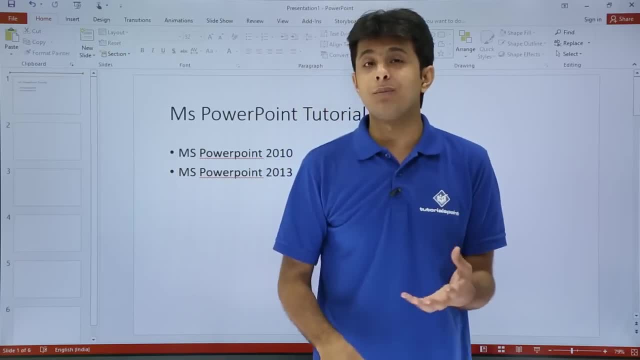 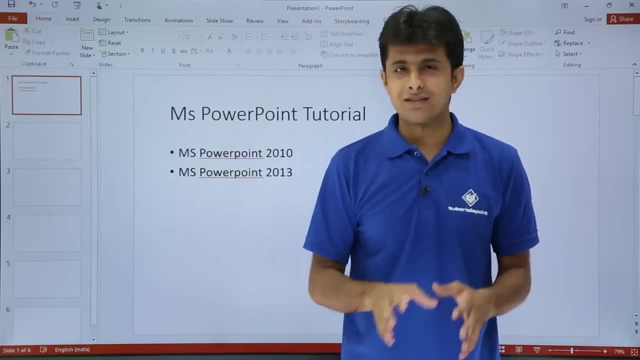 few more options. remove all sections. So all the sections name will be removed and they will be ungrouped basically. So that's it for this video. Thank you for watching. See you in the next video. and you can see all them at together place, right. Similarly, this is how you can create a basic, simple. 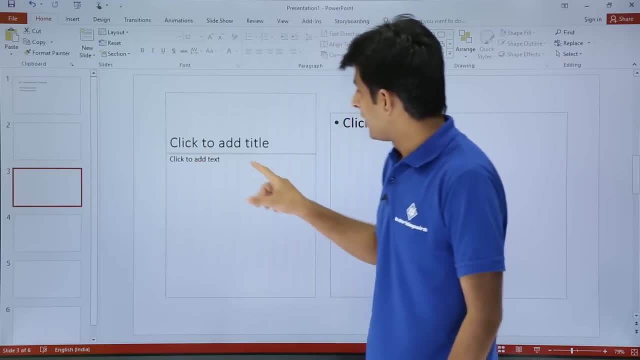 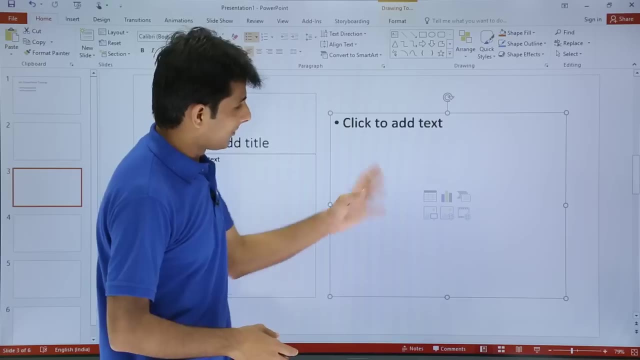 presentation and suppose there's one more which is left here, Suppose I want to. this is a presentation given here slide At this place. if you see there are six options available in this place, You can click here to add text and you can start typing like this, or else what you can do is I'll just